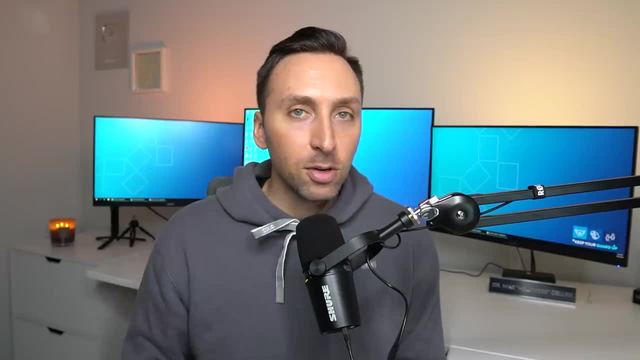 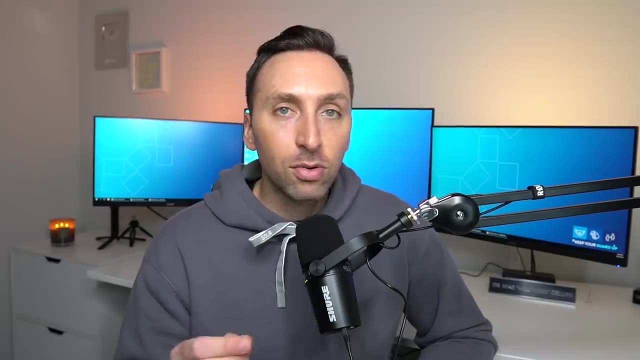 years. Then came three years of residency at Duke University- Shout out Durham, North Carolina, where I used to live- And that took her another four years. In 2014,, she joined the faculty of Duke School of Medicine- And this last line is so crucial to this article- and what? 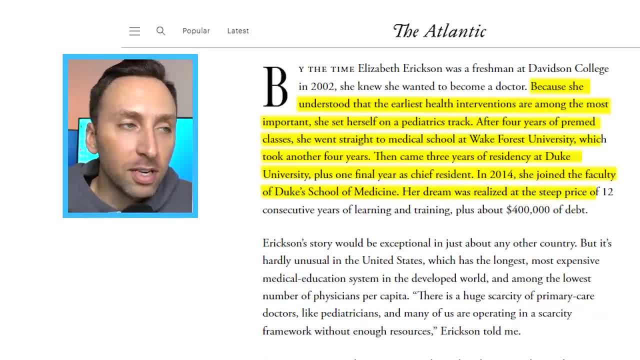 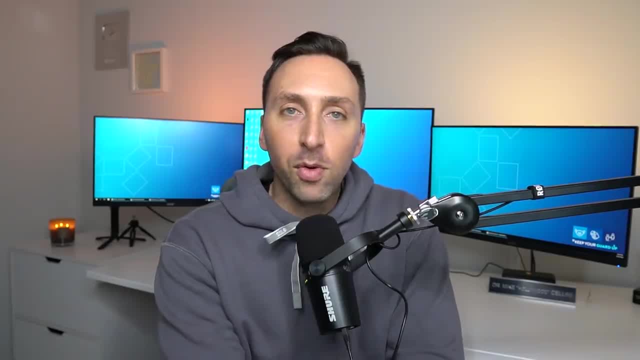 we're going to talk about today. Her dream was finally realized at the steep price of 12 consecutive years of learning and training, plus about $400,000 in student debt. That seems about common for what we've been talking on the channel so far, So let's get into the rest of the article. 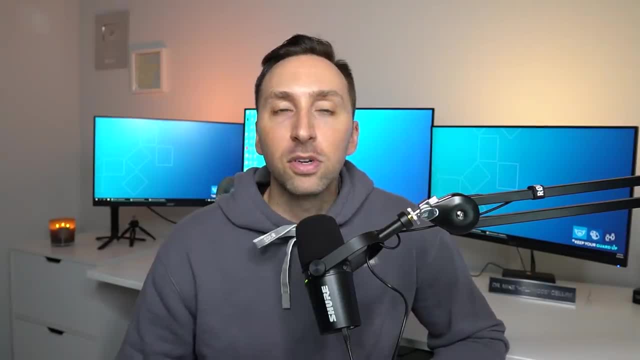 The next part of the article basically talks about how this story would be exceptional in just about every other country in the world except for US. because this article is so important, So let's get into it. This is actually quite common in the US. The US has the longest and most expensive medical 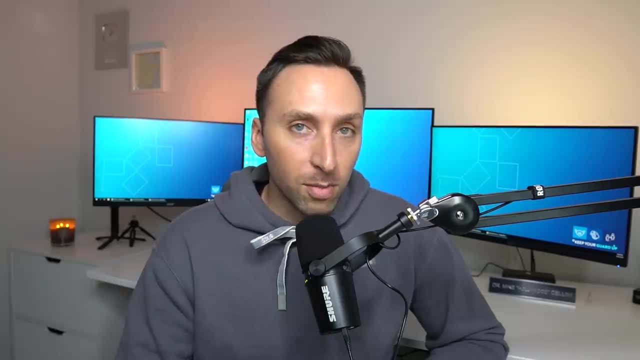 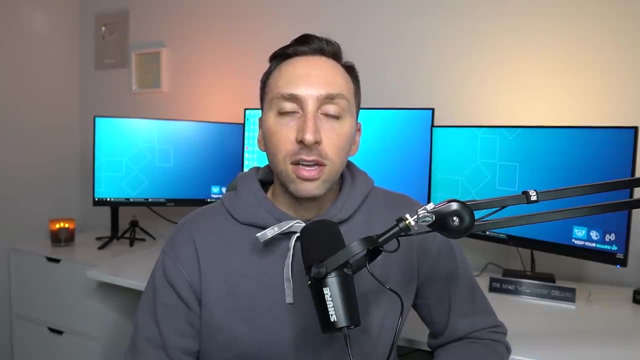 education system in the developed world And, to top it off, the lowest number of physicians per capita, which doesn't make any sense when you say it like that. As many of you may also know, there is a huge scarcity of primary care physicians, and many are operating in a 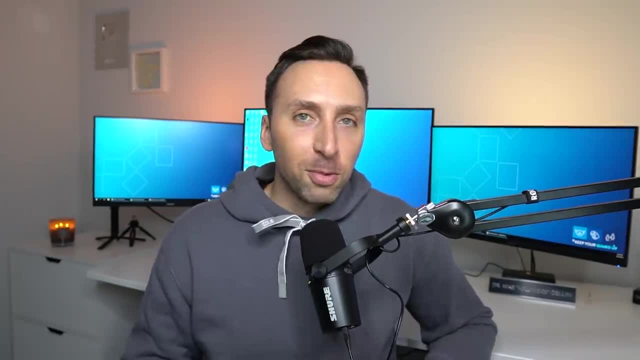 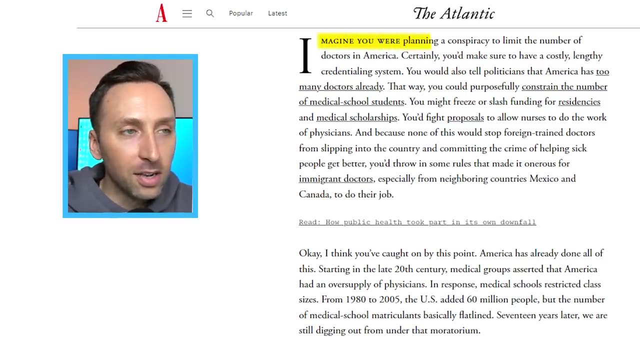 scarcity of framework, with not enough resources. So this is a good part of the article. here We start talking about the nitty gritty of why there are so few doctors in America. So let's start to limit the number of doctors in America. Certainly you'd make sure to have a costly 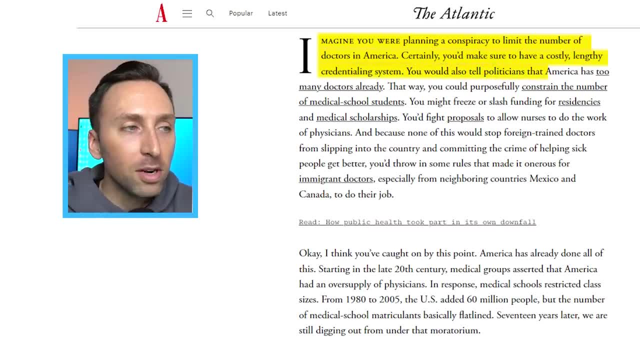 lengthy credentialing system. like we do, You would also tell politicians that America has too many doctors already. That way, you could purposefully constrain the number of medical school students. You might freeze or slash funding for residencies and medical scholarships. You'd 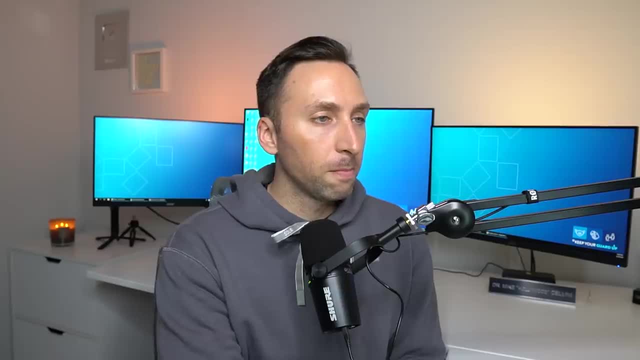 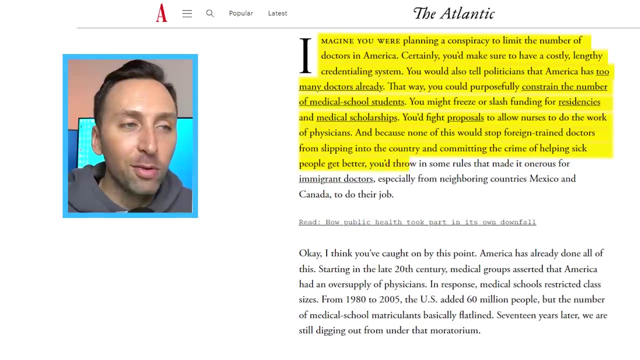 also fight proposals to allow nurses to do the work of physicians, And because none of this would stop foreign trained doctors from slipping into the country and committing the crime of helping sick people get better, you'd throw in some rules. that makes it onerous. especially from neighboring countries like Mexico and Canada. Okay, so let's backtrack a little bit. This article states that in the late 20th century, medical groups asserted that America had an oversupply of physicians. In response to this, medical schools restricted class sizes in these times, From 1980 to 2005,, the US added about 60. 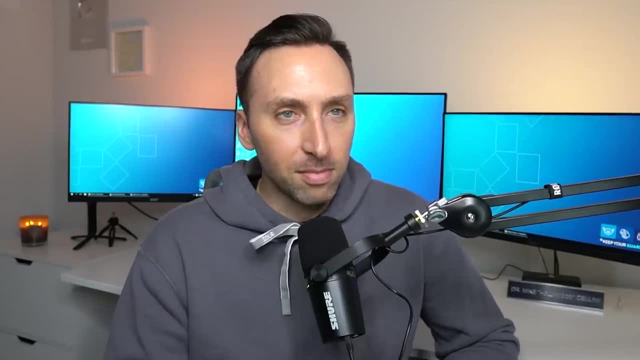 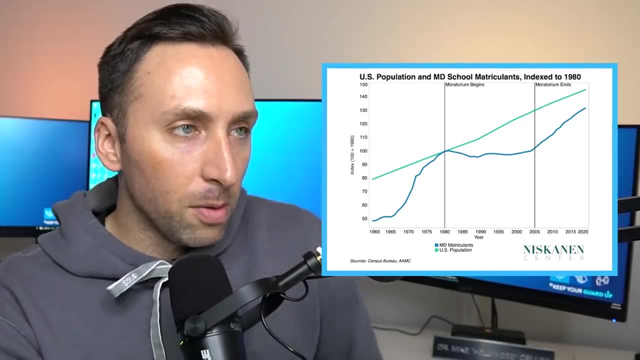 million people, but the number of medical school matriculants stayed the same. 17 years later, we are still trying to climb out of that hole. So let's look at this graph that we show here. So, as you can see here, this shows the US population. 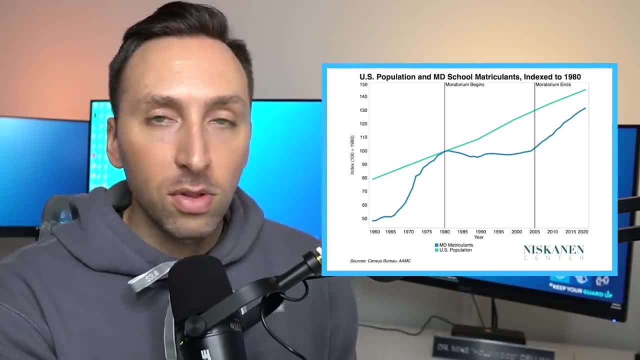 and medical school matriculants, indexed to 1980. The blue line demonstrates MD graduates in the US and the green line represents the US population. As you can see, there's a steady progression of US population with a matching number of doctors until about 1980, when it kind of dipped a little. 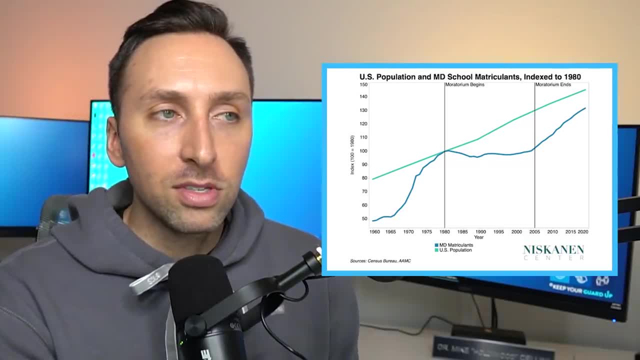 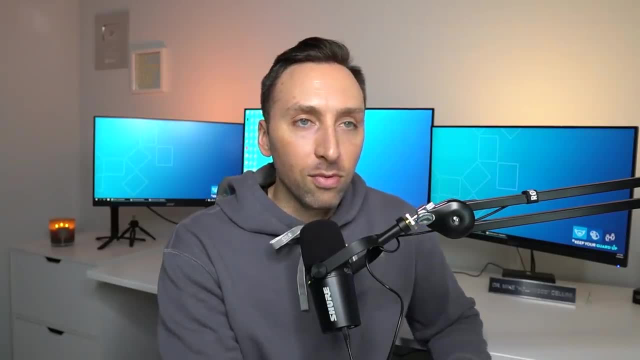 bit and leveled off until about 2005.. And now we're still trying to dig out of that hole and we're not exactly matching the population right now. I think this graph is perfect and it shows exactly what went wrong from 1980 to 2005.. So let's talk about the American education. system for physicians. The US is one of the only developed countries making aspiring doctors get a four-year bachelor's degree, followed by a four-year medical training degree. Most European countries have a six-year continuous program for their physicians, so they are already two years. ahead of us. Then comes residency, of course, which can be anything from three to seven years depending on your specialty, And, of course, our favorite part about the US- medical system, that lovely huge sum of student debt that you're burdened with when you graduate. Now I think I've 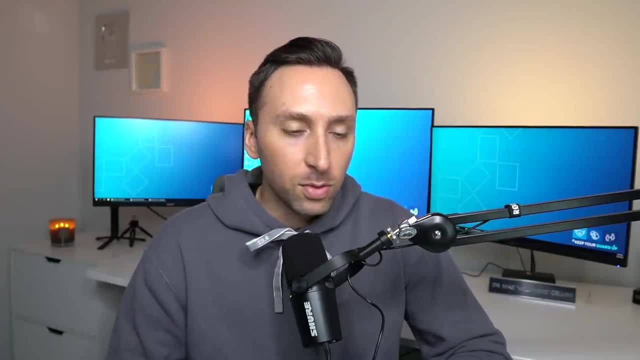 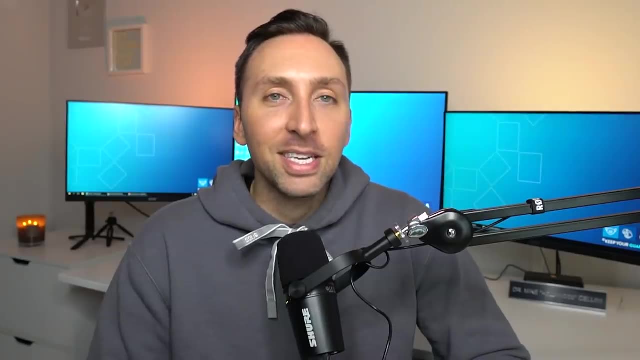 said this on this topic, but I've said it many times, and many medical students finish with somewhere in the neighborhood of $200,000 to even $400,000 plus in student debt, which is insane to think about, And every time I say that statistic it gives me a little chills. So the questions this: 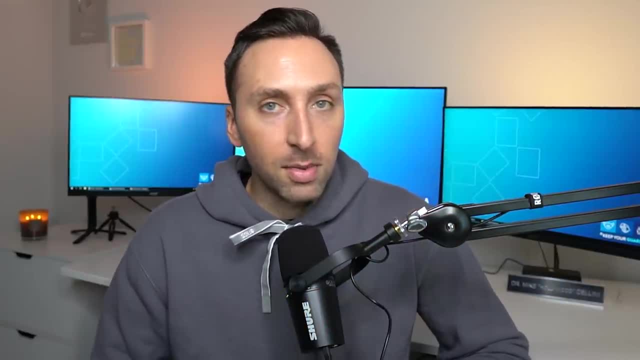 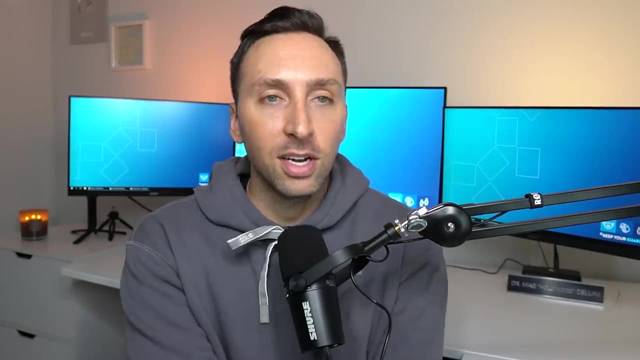 article talks about, and the questions I've had for a long time now are: what is the advantage of extra years of medical training for the US physicians? The author makes a great point here comparing US doctors to Swiss doctors and he says: are American doctors 33% better than Swiss? 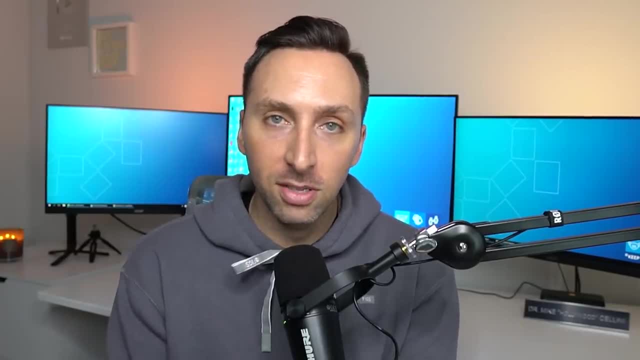 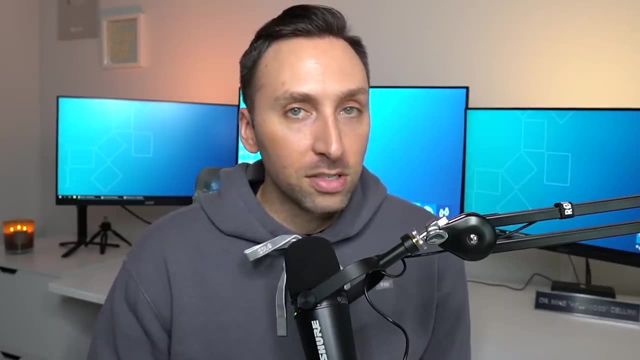 doctors, since we have 33% longer medical education system, which I think is pretty funny. And a nice little aside on this topic is that Americans die earlier than their European counterparts at virtually every age and every income level, And I'll leave a link to that article as well in the 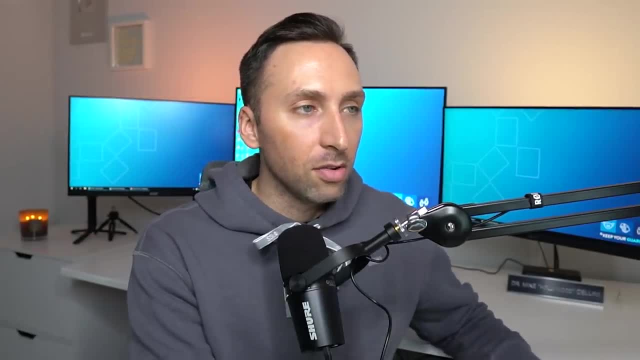 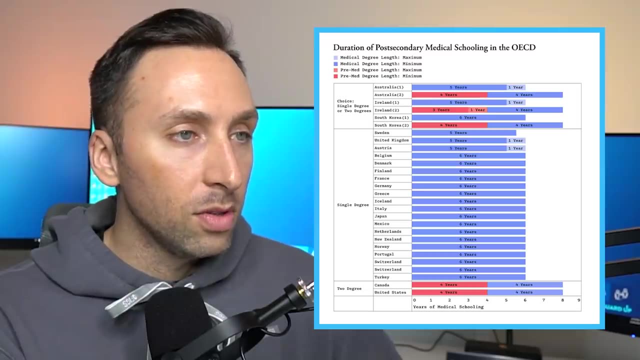 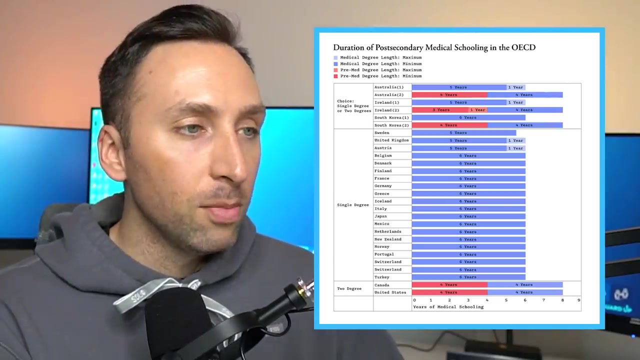 description. Okay, so let's look at this chart for medical education across multiple countries. So, as you can see down here, the United States has a significantly longer track compared to their European counterparts. It takes us four years of undergrad training, four years of medical school, before even going to residency, And most of our European counterparts 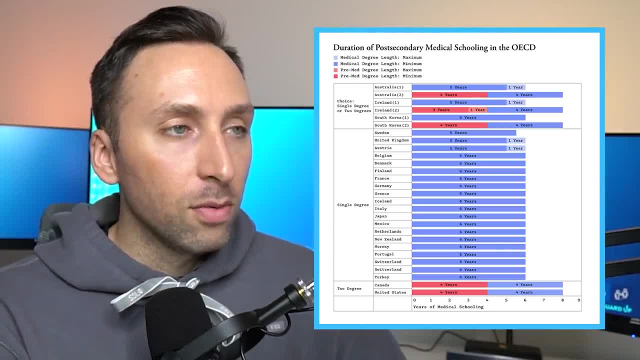 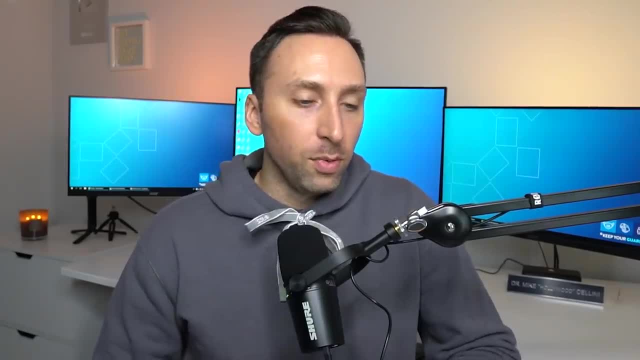 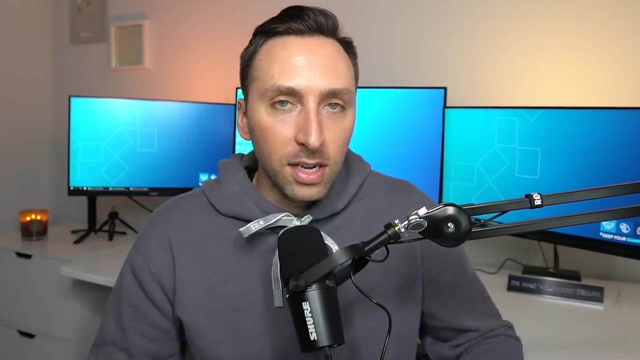 have six years total, with the exception, of course, for South Korea, Ireland and Australia having similar to the American system. So what does this all equate to? when we have medical students who have long education paths and amass a massive amount of student debt, They do what any. 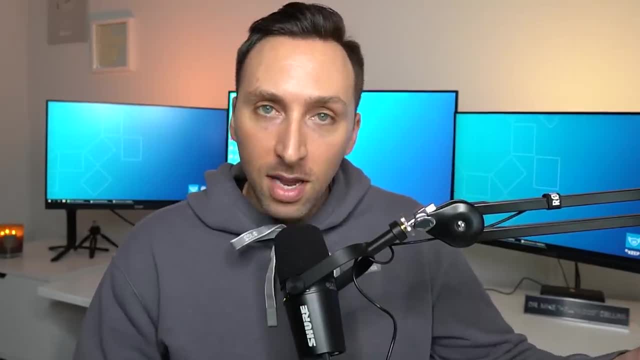 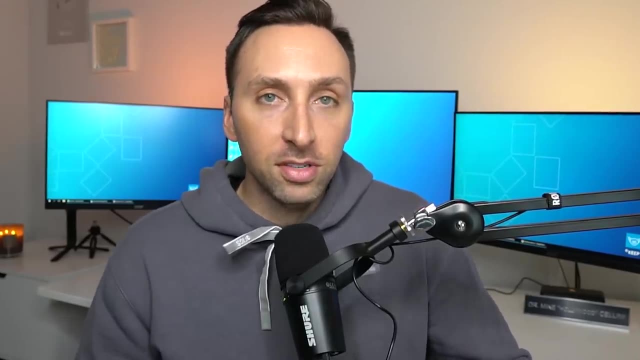 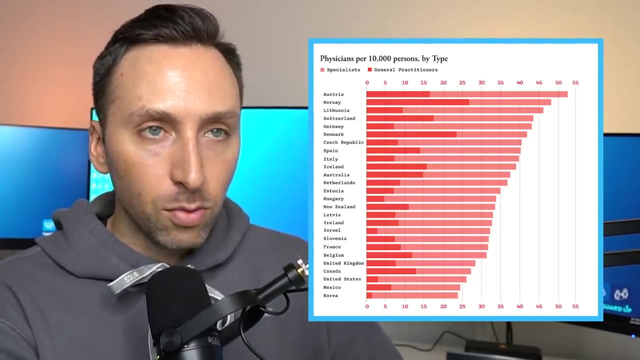 doctor does, and they subspecialize much like I did. So why do we do that? Well, the salaries are limited, which means you can actually pay off your loans. We'll get to this chart in the article as well. You'll see here how the United States has a very small percentage of general practitioners, or 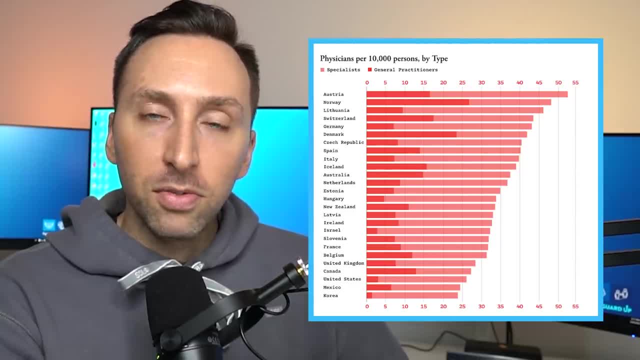 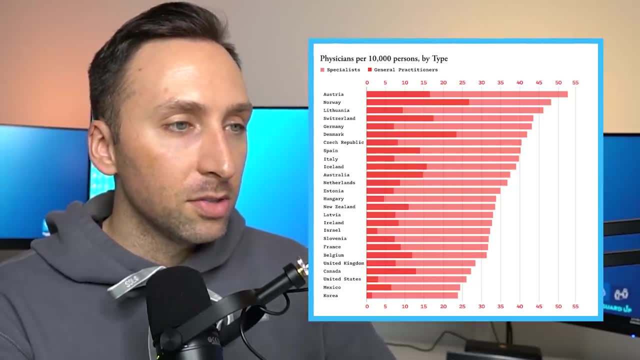 primary care physicians compared to the specialists, in part due to the reasons I mentioned above. So, as you can see, here, United States is way at the bottom and we have a small portion of general practitioners compared to the massive amount of specialists, And this is physicians per. 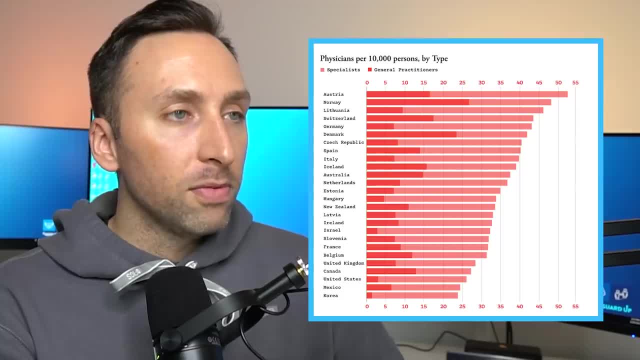 10,000 people, by the way, versus, say, Norway, who is over 50% general practitioners versus specialists. So that's a very small percentage of general practitioners compared to the specialists, and this is physicians per 10,000 people, by the way, versus, say, Norway, who is over 50% general. 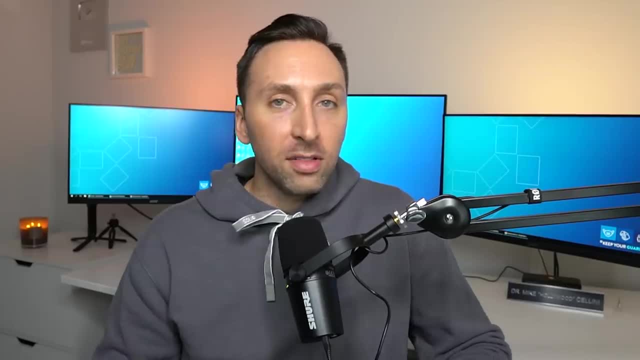 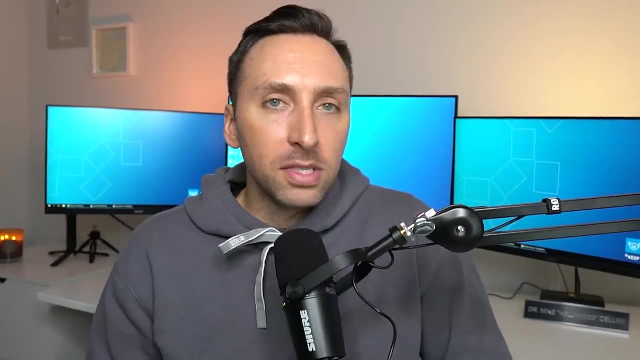 practitioners versus specialists. I think a lot of it comes down to the student debt burden. It's definitely not the lifestyle, because the lifestyle of a primary care physician is pretty good. It's the usual eight to five job. I don't think a lot of them take call. Some may. 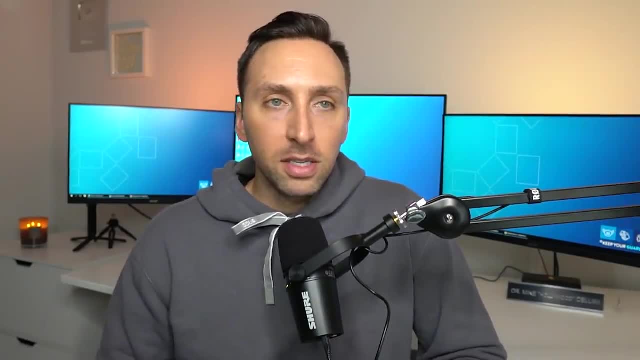 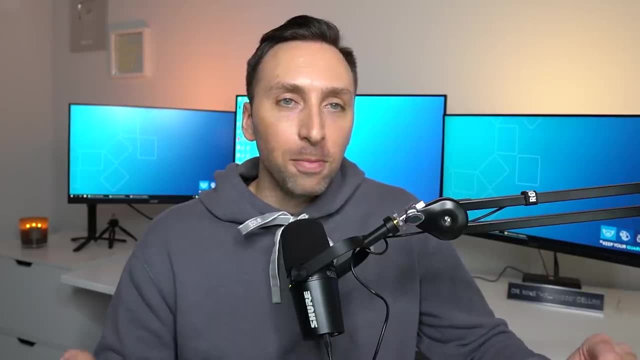 take call in the hospital, but most of it is clinic-based, outpatient-based and not that bad. Well, I say that relatively because I know their burden with seeing an enormous patient load. but, all things considered, if the patient load was down, you can practice how a primary care physician 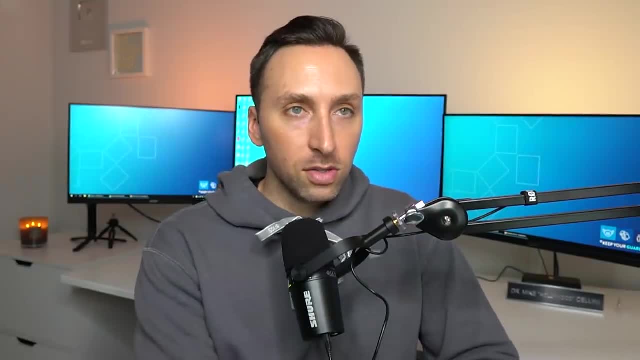 is supposed to practice. It's a pretty good lifestyle. Now this article goes on to talk more about how some doctors actually object to more competition for the same reason that homeowners object to more local construction. Docs are afraid of competition because it ultimately cuts into their piece of the. pie. However, if you look at it a different way, more docs in one region can actually make life better for that particular doctor, because they're not burdened with longer hours or seeing excessive amounts of patients, which improves the quality of life and prevents burnout. I love this line. from the article. here It states: doctor burnout and brutal 16-hour shifts for residents. I love this line from the article. here It states: doctor burnout and brutal 16-hour shifts for residents And MDs aren't necessary tests of willpower. They're just the inevitable result of not having 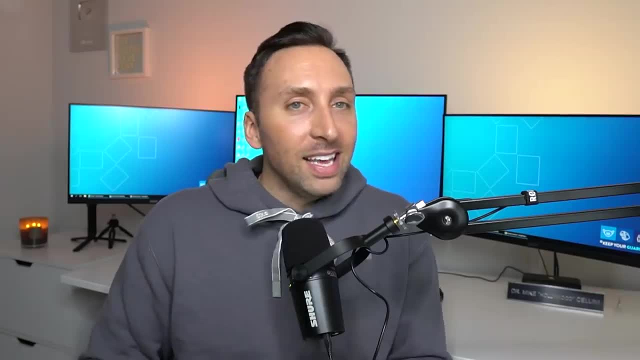 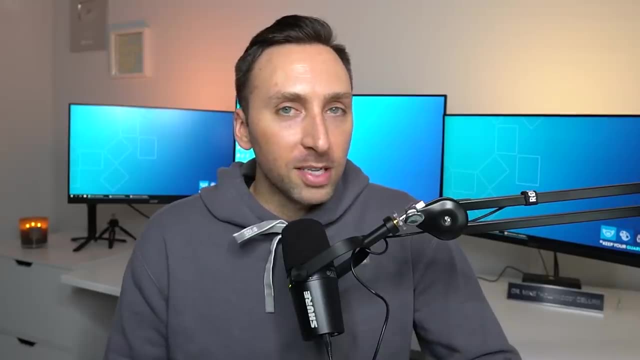 enough people to do the work that today's hospitals demand. That basically hits the nail on the head in every possible way. So it's kind of a rhetorical question: but why do we need more doctors? Well, for one, the pandemic has proven a significant burden to the healthcare. 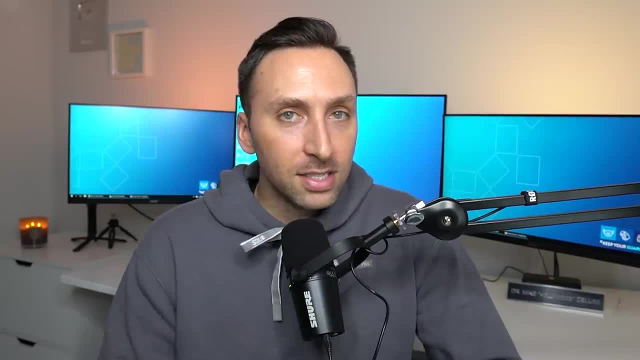 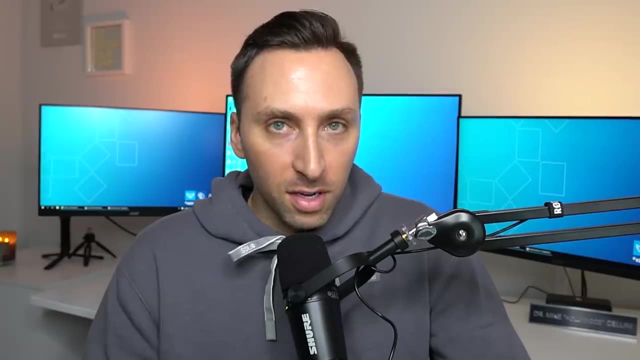 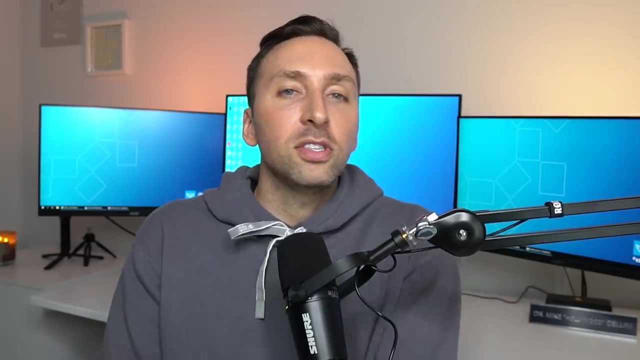 system and, most importantly, healthcare workers. And regarding the census, which states: in the next 12 years, we will have more senior citizens than children in America for the first time in history, I think we're going to need more doctors. So what's the solution to this problem of so few doctors in America? Well, I think it's obvious: We 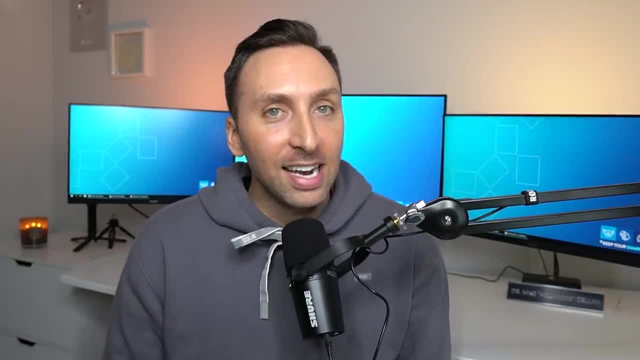 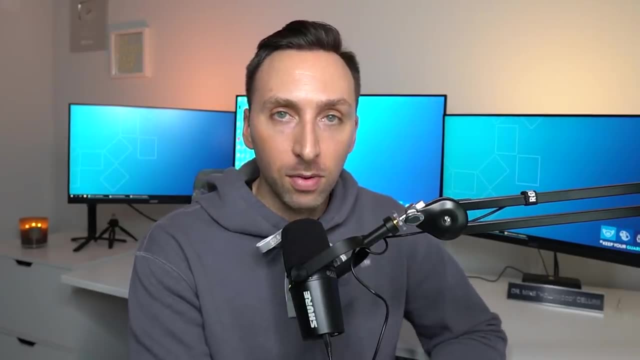 just create more doctors. It's that easy. Okay, so it's obviously not that easy, as this is clearly a deeper systemic issue. In the article, they posed this question to a healthcare policy analyst, who stated the following: The first thing I would do is expand the residency system so that more 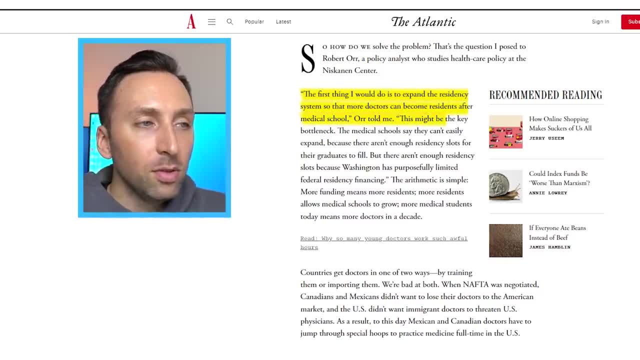 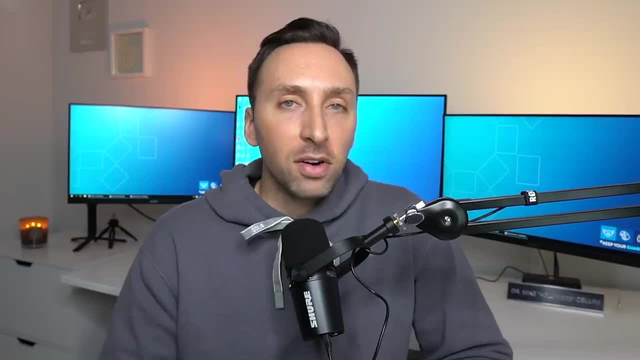 doctors can become residents after medical school. This might be the key to the bottleneck. Medical schools say they can't easily expand because there aren't enough residency slots to fill for their graduates, which is very true, And every year we have the problem where we have too many. graduates for residency spots, and some medical graduates, aka doctors, do not match into residency, which leaves them residency-less. Imagine having gone through eight years of training only to not be able to match into a residency program because there aren't enough spots, And ultimately they may have to scramble into a residency that they don't want to do just. 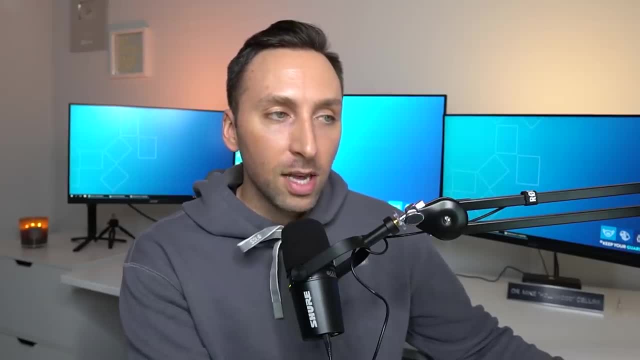 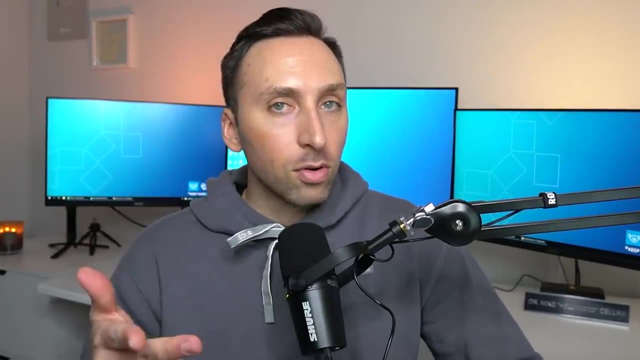 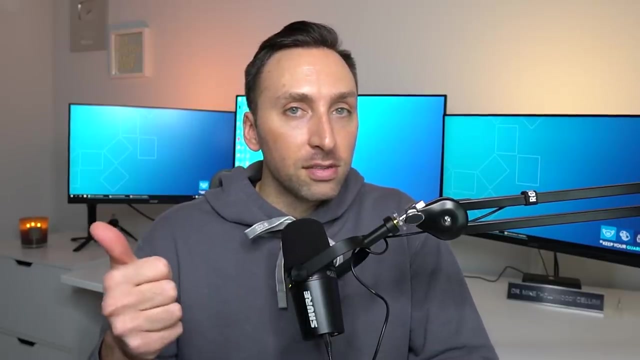 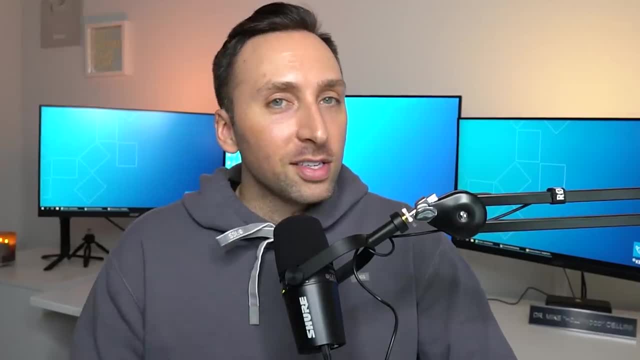 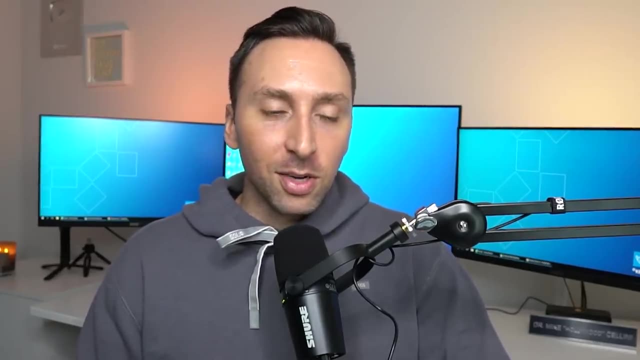 as doctors in rural or underserved areas. but we're not going to touch on that topic because it's a little too dicey right now, at the moment, and I'm sure people in the comments would go a little crazy once we start talking about that. So that's just something we're not going to touch on. 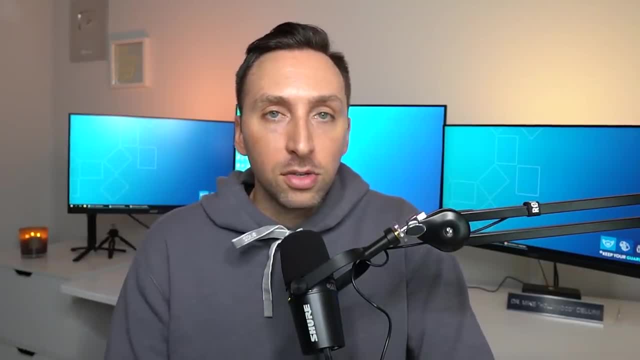 today. So how else could we fix this problem? Well, we could extend care to underserved areas via legal telemedicine. but the problem is we have to get reimbursement from the government for the physicians doing those telemedicine consults, because during the pandemic it was. 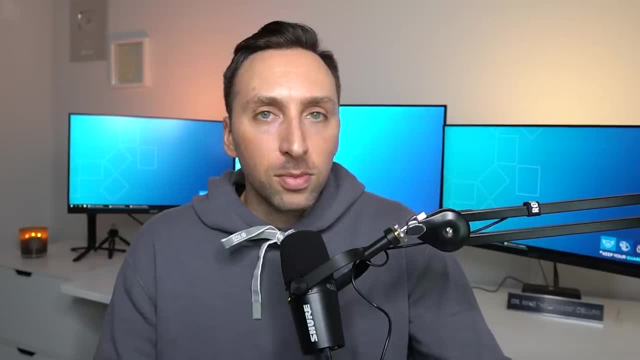 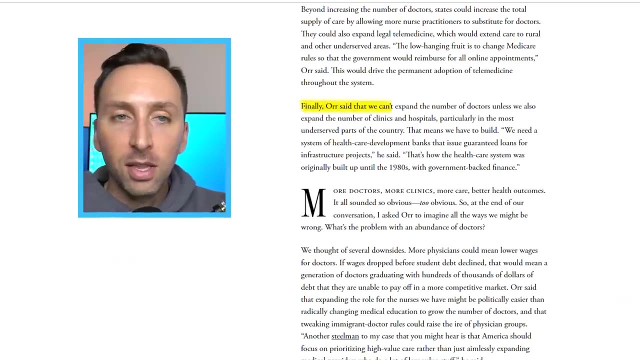 allowed, but it's not really 100% so far. So there's more work to be done in the telemedicine slash reimbursement space. Another good point this healthcare policy analyst stated is that we can't expand the number of doctors unless we also expand the number of clinics and hospitals, especially to 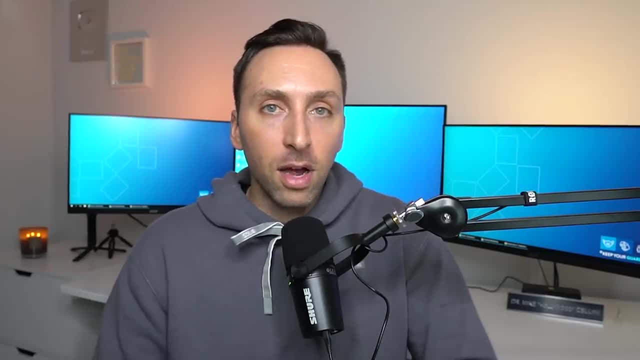 the underserved parts of the country. Basically, we have to have more funding for hospital infrastructure. So, in conclusion, this all seems really simple: More doctors, more healthcare infrastructures and more care equals better healthcare outcomes. But, as always, we have to crawl before we run. 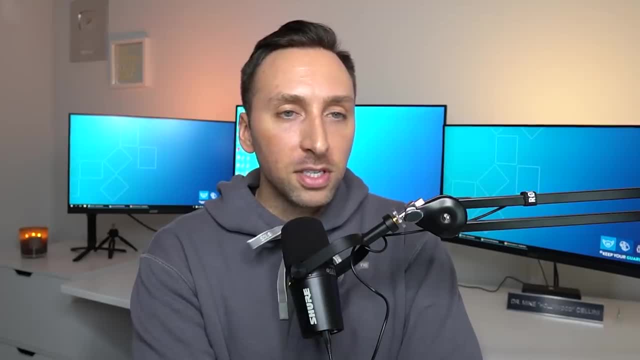 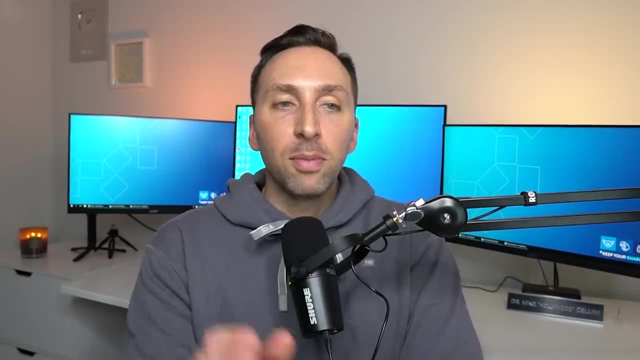 The article makes a great point here and states that if we put an influx of physicians into society, then we lower wages for physicians, which is okay. But the problem we would face is that we'd have to ensure that the wage drop occurs before student debt declines, because then we would have a bigger issue altogether. If wages drop before student debt drops, then we have doctors making low wages with no way to pay off their massive student debt burden, And then we have a whole other problem, Speaking of which, why the heck are universities and medical schools charging so?